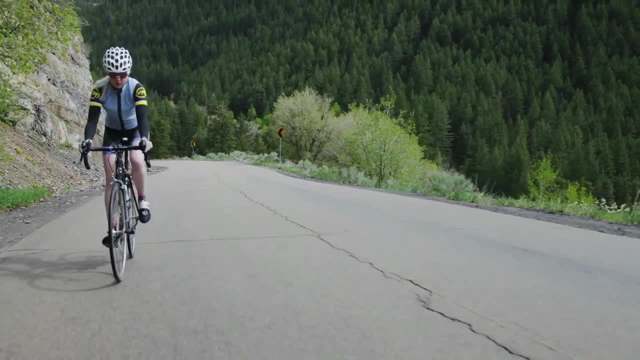 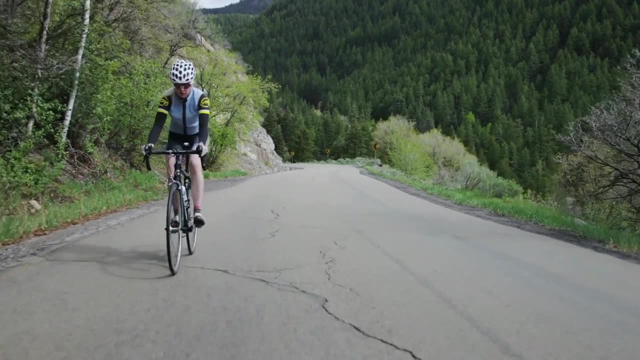 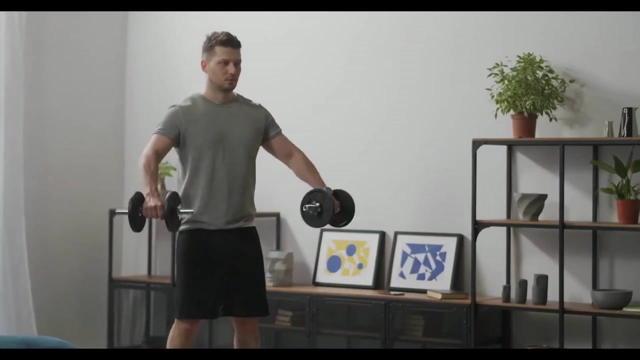 This cyclist is applying work to the bike in order to produce power which propels the bike up the hill. Let's take a look at the relationship between work and power. Welcome to MooMooMath and Science. What do these three video clips have in common? 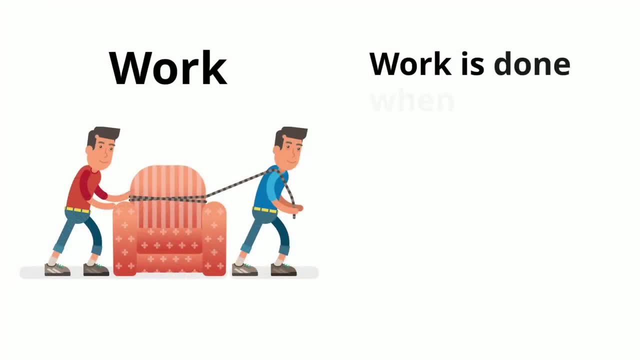 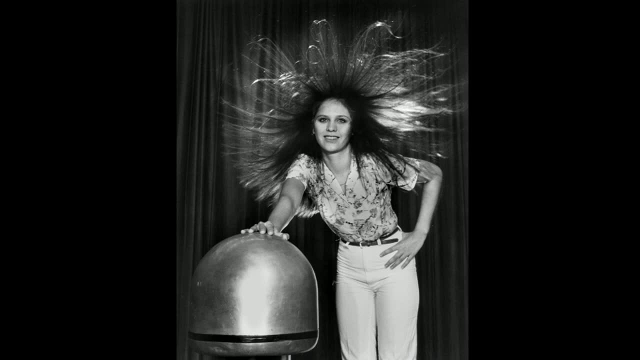 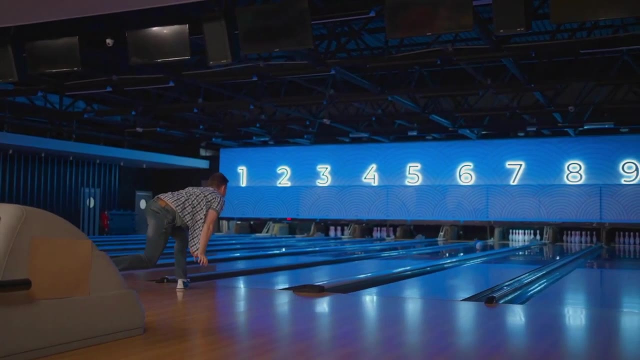 They are all examples of work. Work occurs when a force causes an object to move in the direction of the force. Work transfers energy from one object to another. Let's take a look at an example. Force is being applied to the bowling ball by the bowler. 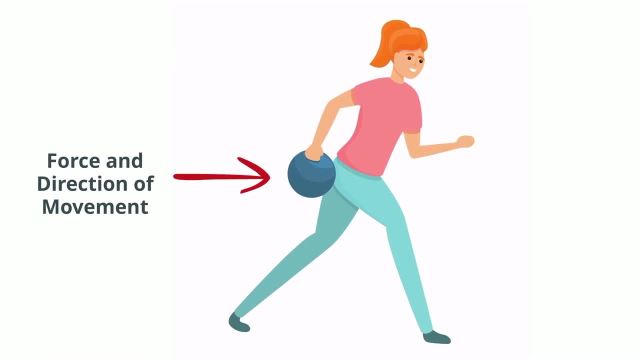 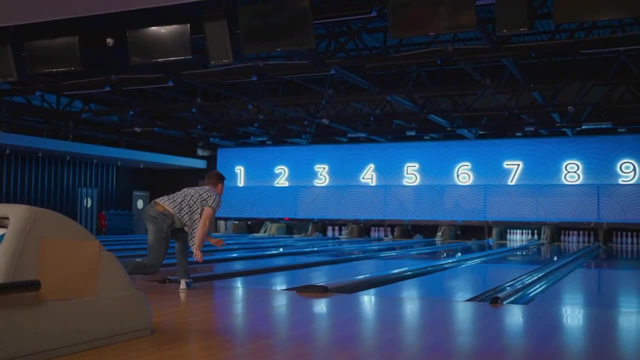 The force is applied in the direction that the bowling ball is moving. When he releases the bowling ball, he will no longer be doing work because he can no longer apply force to the bowling ball. Applying force does not always result in work being done. Imagine: 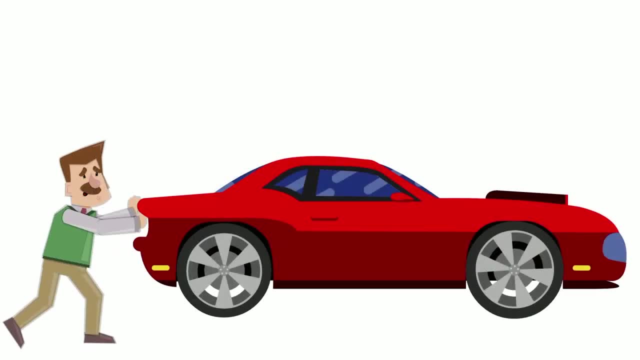 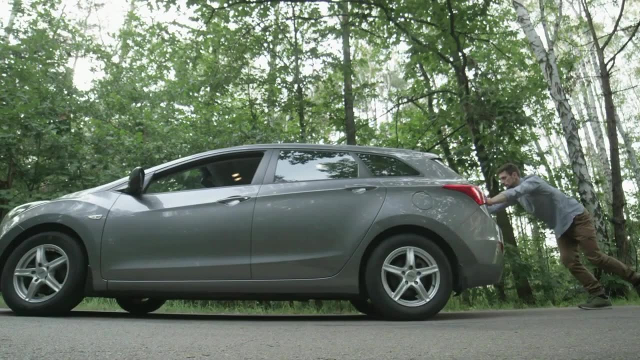 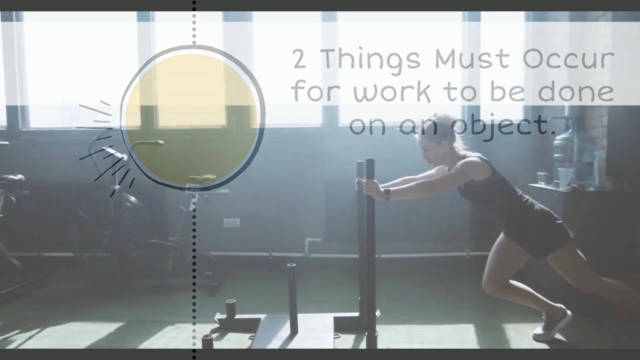 you are trying to do the following: You push and push, but the car won't move. Because there is no movement, there is no work. that is done As soon as the car moves, work is being done. Two things must happen for work to be done on an object: The object must move as the 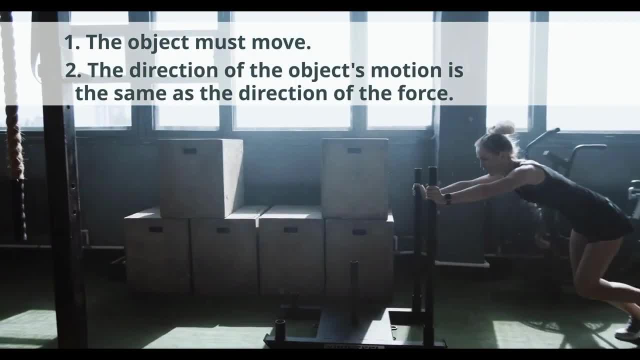 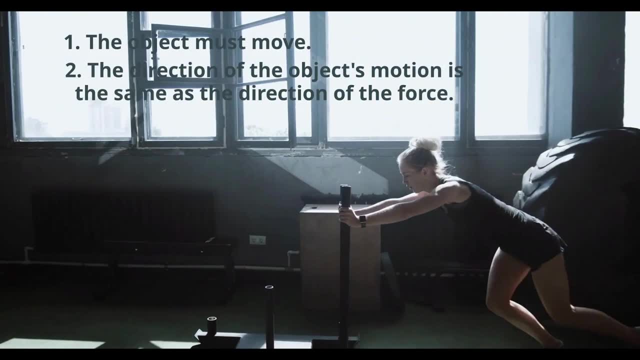 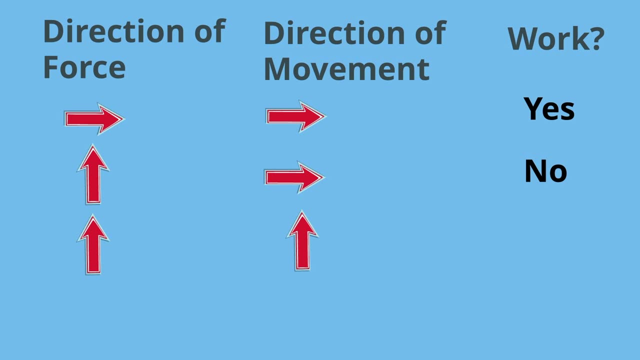 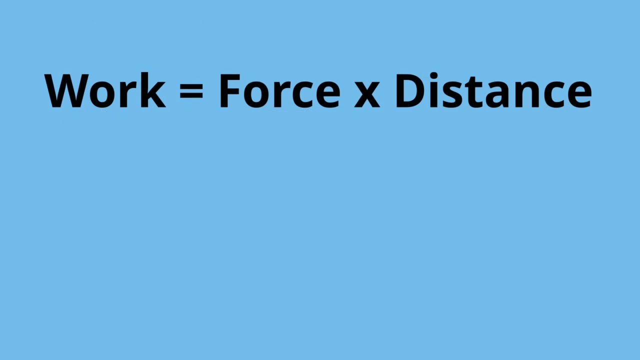 force is applied and the direction of the object's motion is the same as the direction of the force. Let's take a look at a couple of examples and non-examples. The force is applied to the object by the distance that the object moves. The formula is equal to: w equals F times d. 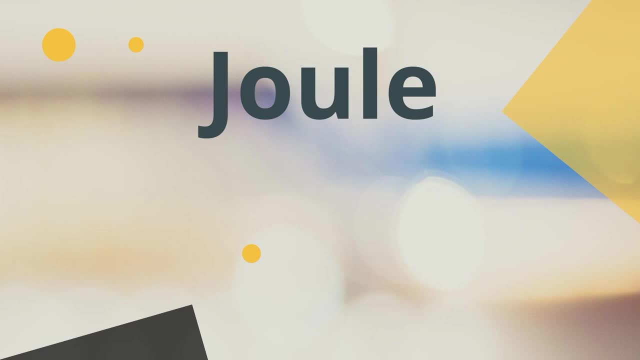 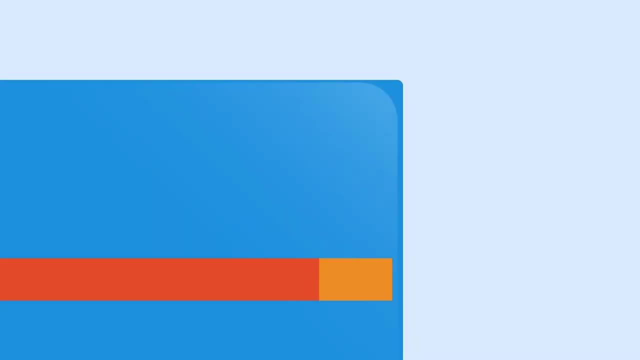 Work is expressed in joules, which is the amount of work done by a force of one Newton. the mass of the force. The mass of the force is given by the force of the force of the acting through a distance of one meter. Now let's talk about how work relates to power. 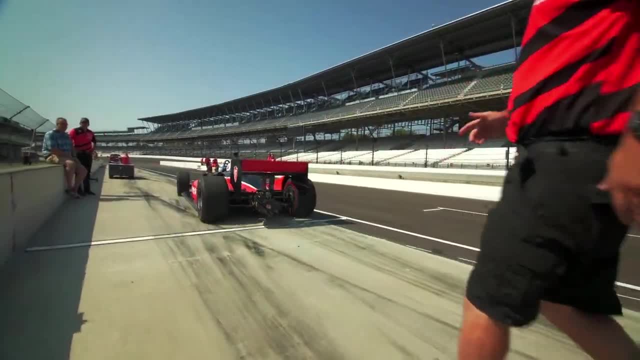 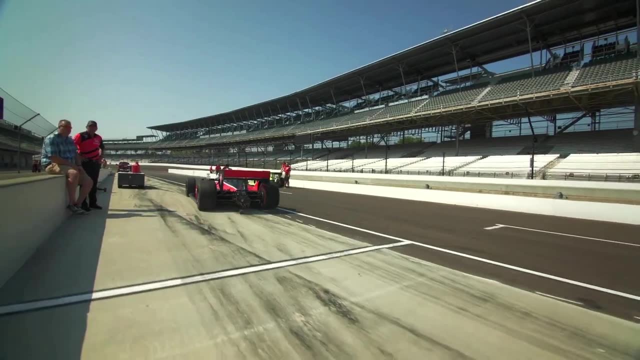 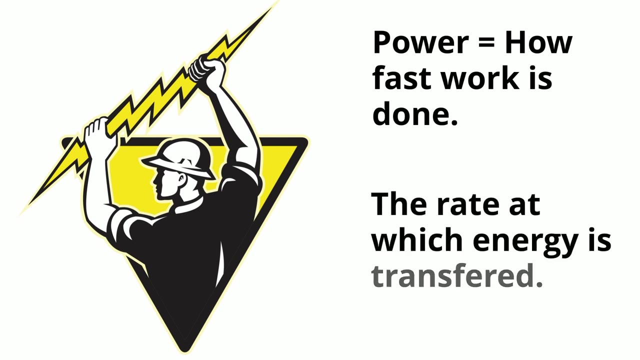 Which of these two cars is more powerful, This race car or the friendly family car? Yes, the race car, But what are you measuring when you're talking about power? You can think of power, of how fast work is done or the rate at which energy is transferred.